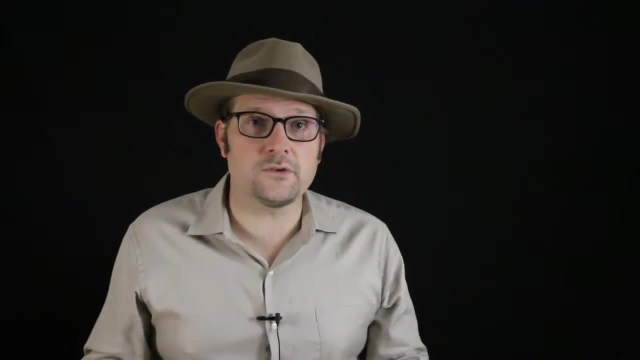 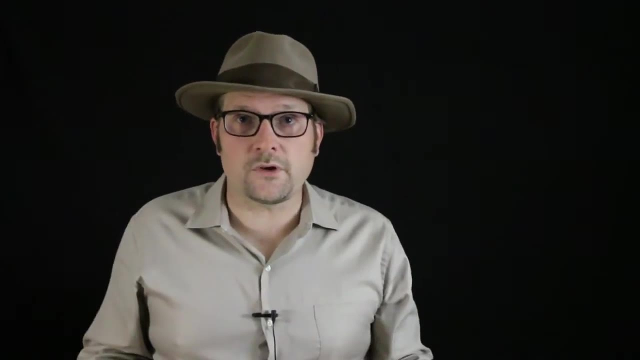 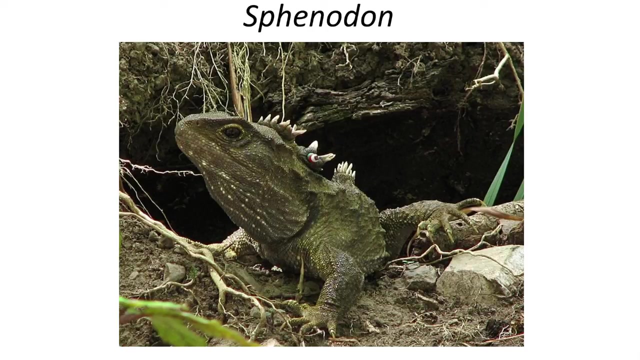 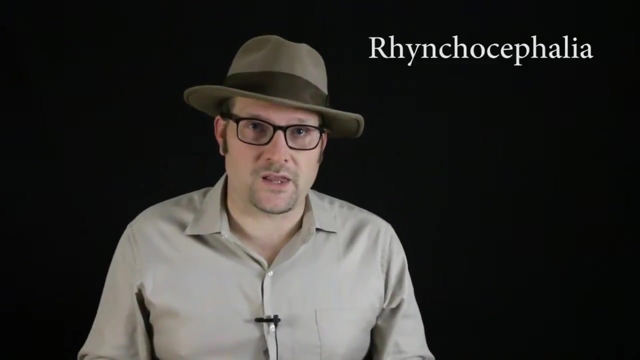 populations, Although populations have been reintroduced onto the main islands recently in protected wildlife sanctuaries. These unusual animals are called the Tuatora, scientific name Sphenodon, and they belong to an ancient lineage that extends all the way back to the Triassic called the Rhynchocephala. 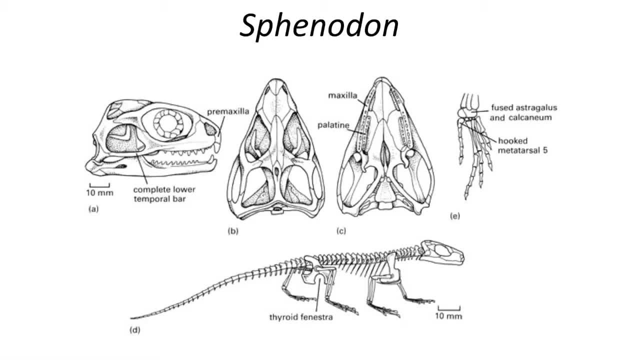 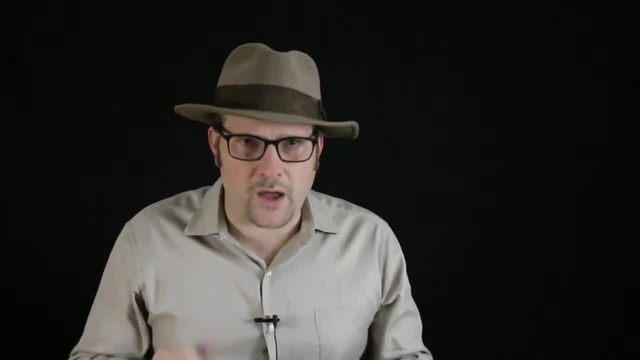 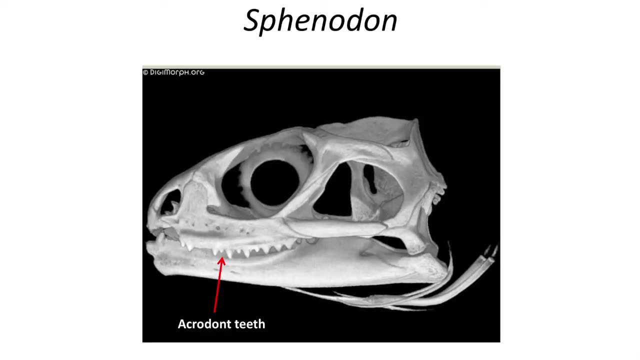 Now let's take a look at the skull of a Tuatora and see what primitive features the animal has that makes it unique from other lizards. The first thing we notice in the skull is that the Tuatora has acrodont teeth. 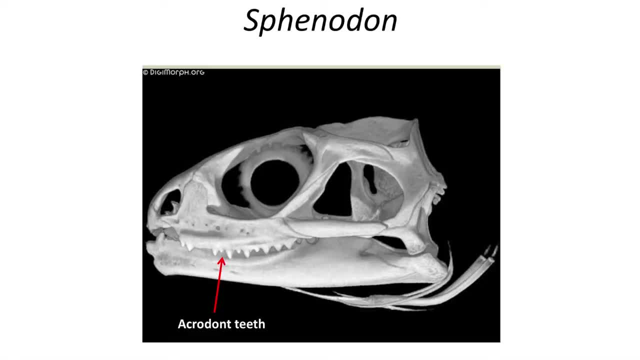 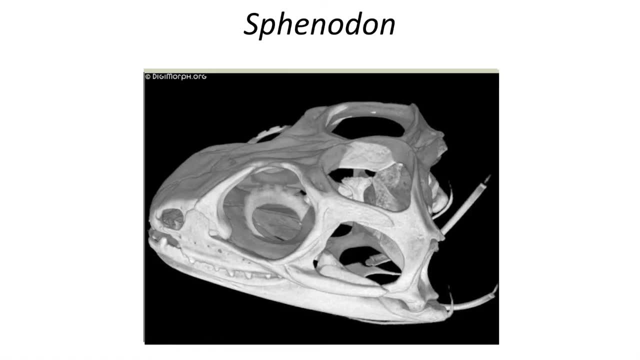 These are teeth that bud onto the bones in the jaw rather than being nested in sockets, like the archosaurs and mammals have. The skulls have two rather large toes, Temporal fenestra, which are well pronounced, making this lizard very clearly a diapsid. 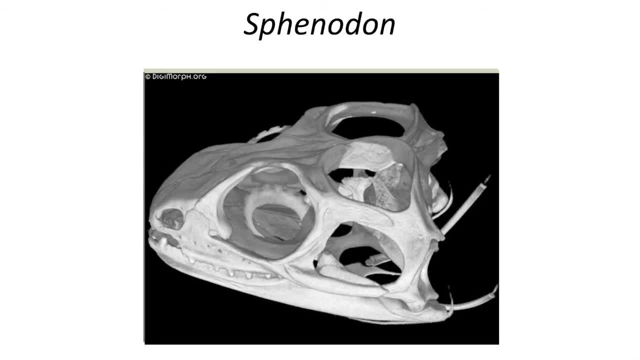 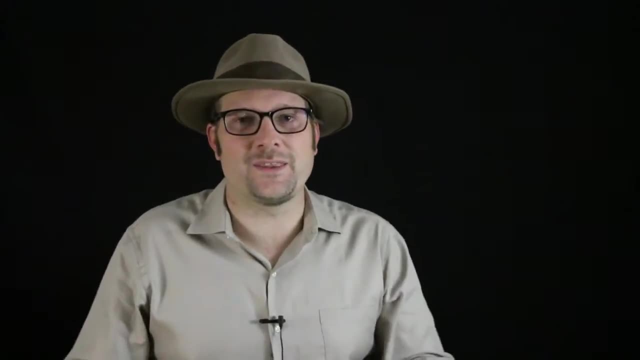 reptile. The anterior snout lacks any fenestra, with a simple narrow opening for the nostril. You also notice a scleral ring which helps support a rather large and unusual looking eye. Now, why are the Tuatora not included within the Squamata with the other lizards? 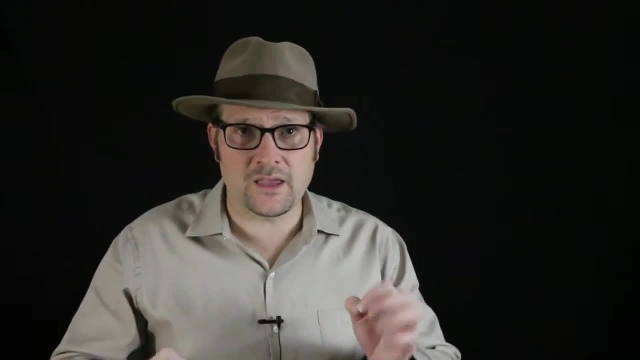 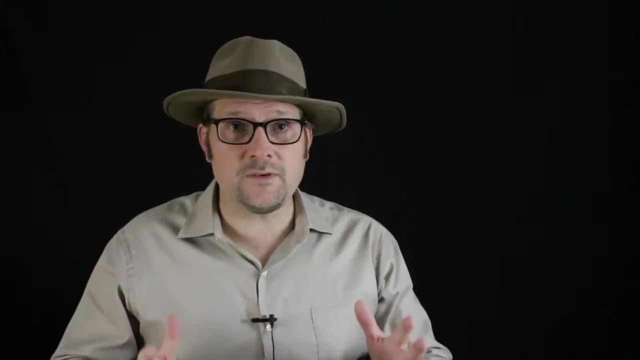 Well, it has to do with something that it likes And that something is called cranial kinesis, which is found in lizards, snakes and even mosasaurs. These are giant marine lizards. So what is cranial kinesis? 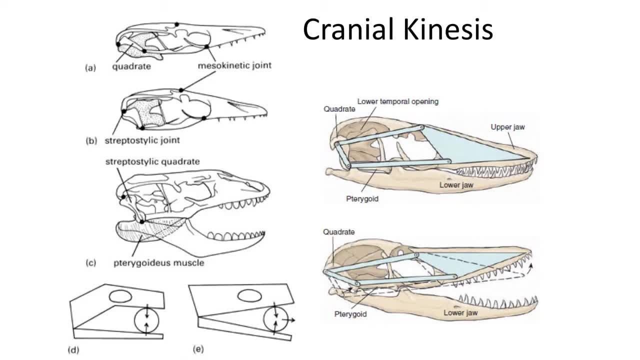 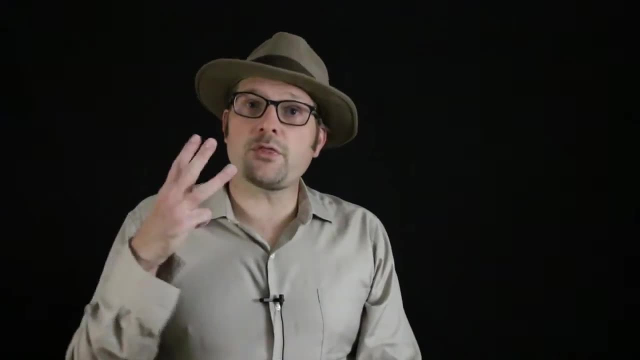 Cranial kinesis is additional joints within the skull that support additional movements of bones in relationship to each other, And lizard, snake and mosasaur skulls are highly mobile and these joints facilitate the eating of prey. There are three principal joints in the Squamata skull. 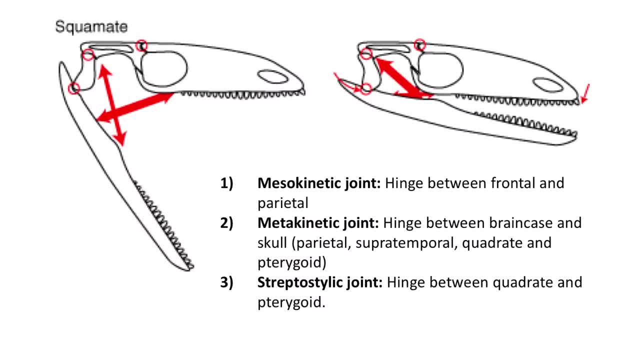 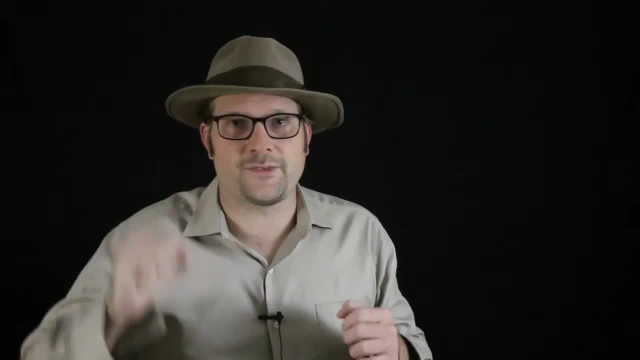 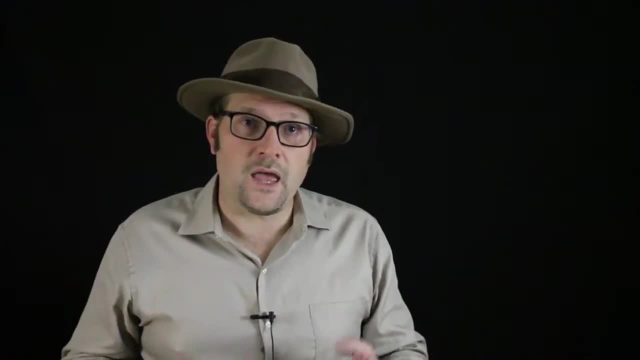 The first is called the mesokinetic joint, which is a hinge between the frontal and parietal. This joint allows the snout or front half of the skull to hinge downward during a bite, giving it a less wedge shaped bite and more downward force for crushing and holding onto. 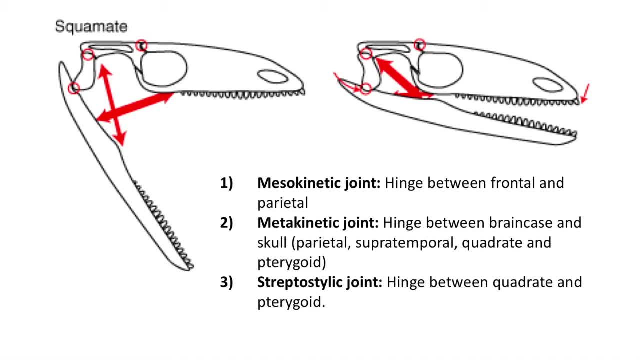 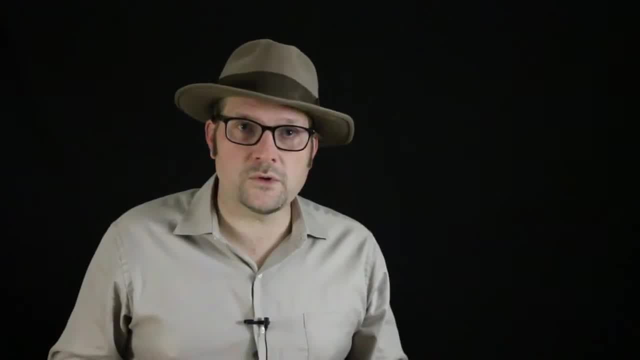 prey. The second joint is the metakinetic joint, which is a hinge between the brain case and the skull, And finally the streptostylic joint, which is between the quadrate and pterygoid. The joint pushes the jaw forward during the bite. 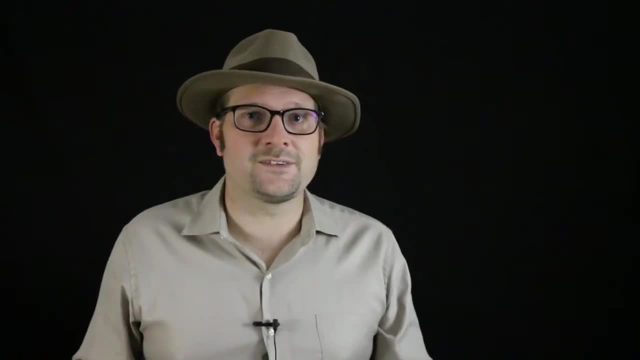 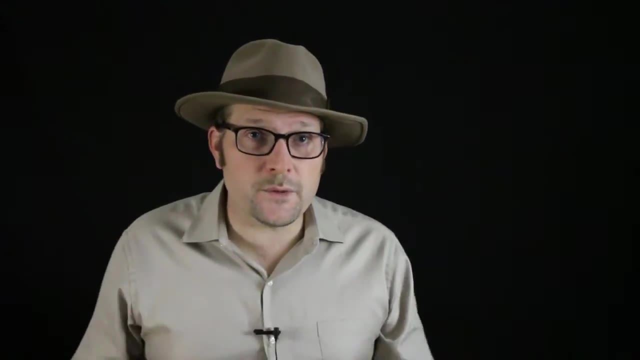 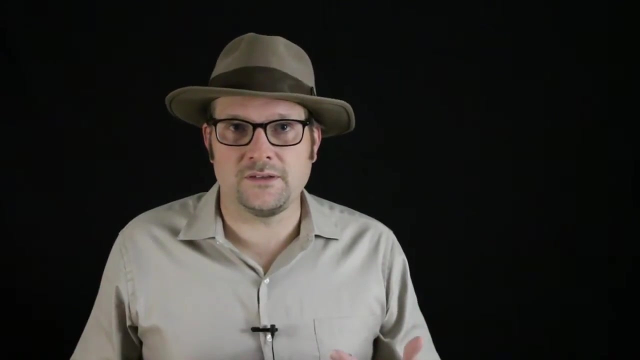 There is considerable veneration in the cranial kinesis among lizards and snakes, with most having stereostylic joints, while the primitive clade, the iguana, which includes the iguana, lizards and chameleons, lack the mesokinesis joint between the frontal and parietal. The most mobile lizard skulls are found in the Varanidae family, which are believed by some researchers to be the most closely related lizard group to snakes, which have very mobile skulls which include even additional joints in their skull. This is because the most mobile lizard skulls are found in the Varanidae family. Most groups of lizards originate during the middle and late Cretaceous period, and the most mobile lizards are found in the late Cretaceous period. The most mobile lizards originate during the middle Jurassic, including geckocata skinky. 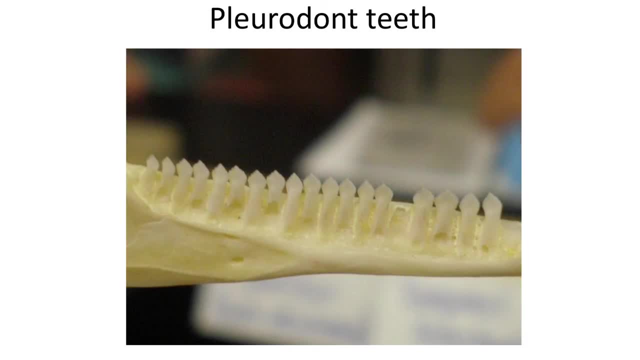 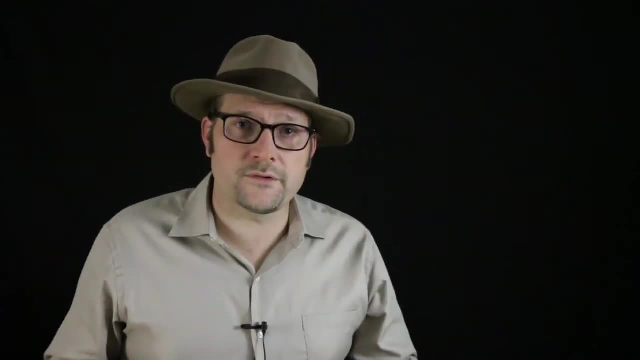 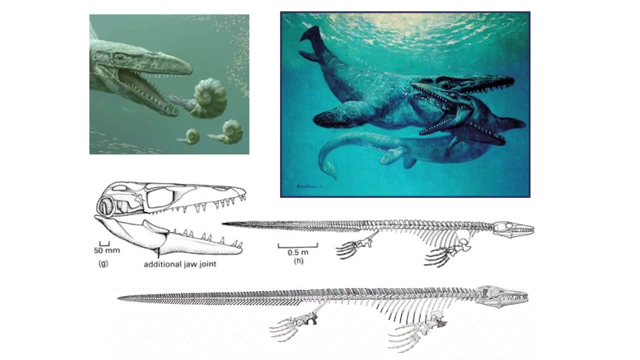 amorphous, which exhibit pleurodont teeth, as well as a diverse group of angiomorphs which include the varanids, such as the Komodo dragon, as well as large marine lizards called mosasaurs. There are a few legless lizards, in particular a genus in the skink family which tend to 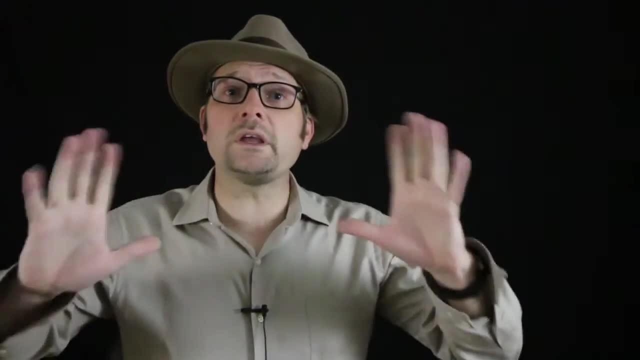 retain the legs. The most mobile lizard skulls are found in the Varanidae family, which include many mobile lizards which include a genus in the skink family, such as the Komodo dragon, as well as a diverse group of angiomorphs, which include a diverse group of angiomorphs such as the. komodo dragon, which tend to retain the legs To the completely legless Amphisbanians. The Amphisbanians are tiny subterranean worm-like lizards which have a growing fossil record going back to the base of the Paleocene. They have an unusual biogeography today, including Africa, South America and Central America, puzzling scientists on their possible post-breakup of Pangea origins. Yet they have a near-global record of life and death. They have a near-global record of life and death. 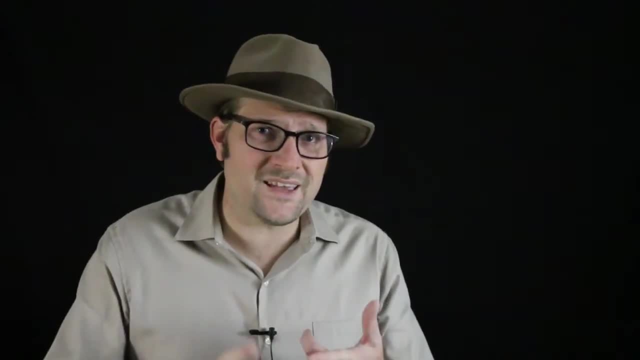 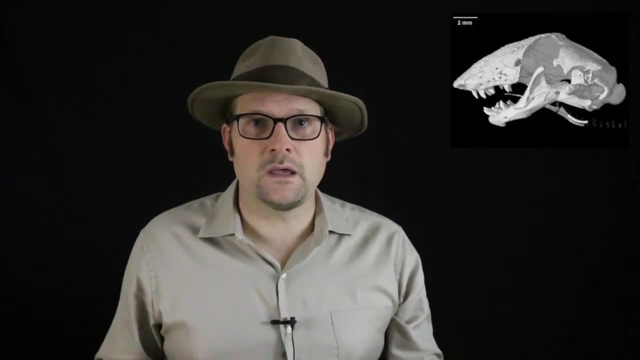 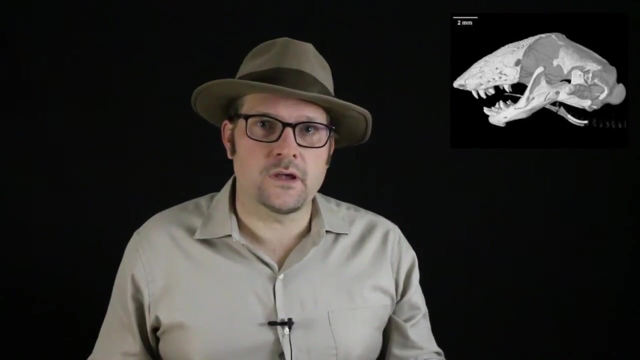 global distribution. despite their late origin and subterranean lifestyle, The skulls of Ampsus bainids lack cranial kinesis and is composed of a single, tightly fused skull. They are tiny creatures. they eat worms and other invertebrates underground and resemble. 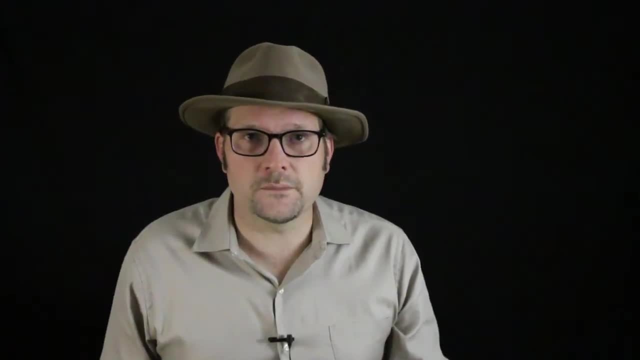 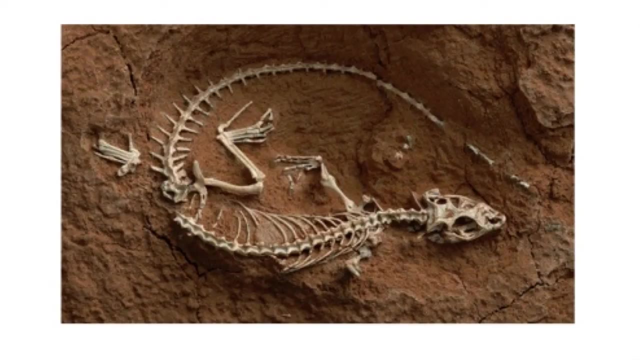 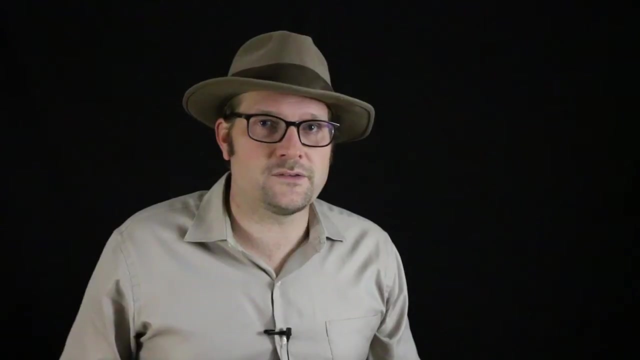 in many ways the Sicilian amphibians. The fossil record of lizards from the late Cretaceous and early Cenozoic is particularly good, indicating the success of the group through the end Cretaceous extinctions. But some groups did not go extinct, while others survived and quickly diversified in the early Cenozoic. In fact, like mammals and birds, lizards also likely underwent a major diversification following the end Cretaceous extinction, And new fossil discoveries in the early Cenozoic are also likely to be found in the early Cretaceous.